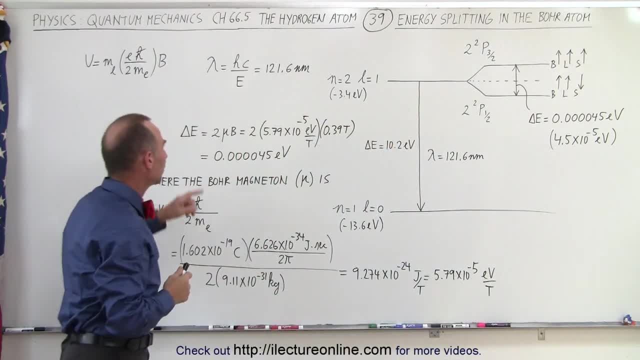 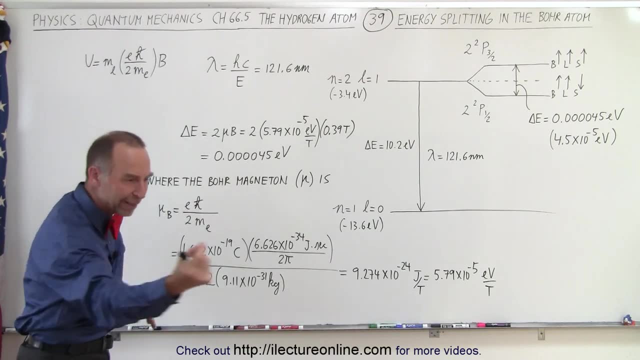 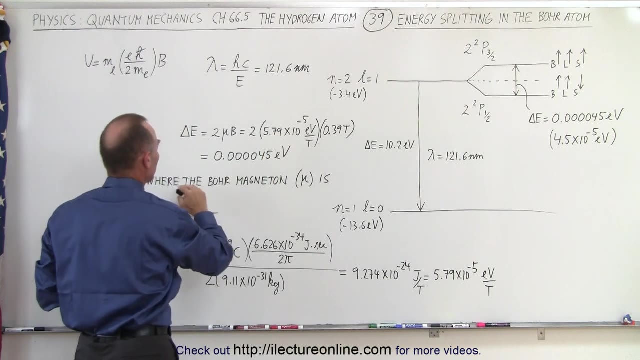 difference in the energy level. Well, the difference in energy level will be twice mu times B. Now, what's mu and what's B? Well, B is the magnetic field caused by the orbiting electron, which is about 0.39 teslas. Mu here represents what we call the Bohr magneton. It's the quantity 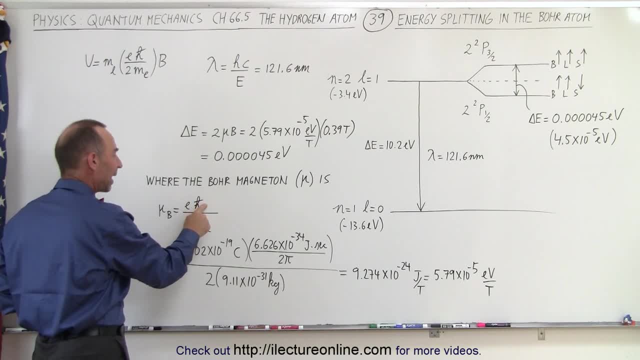 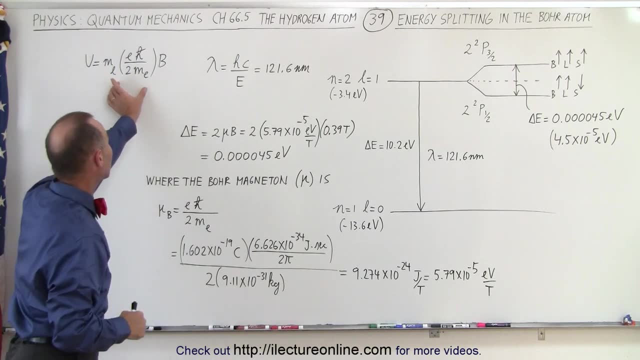 that's defined by the charge on the electron times, Planck's constant divided by 2, pi divided by 2 and divided by the mass of the electron. Now, this quantity here fits in the equation that calculates the energy caused by this interaction between the B field, caused by the orbital motion of the electron. 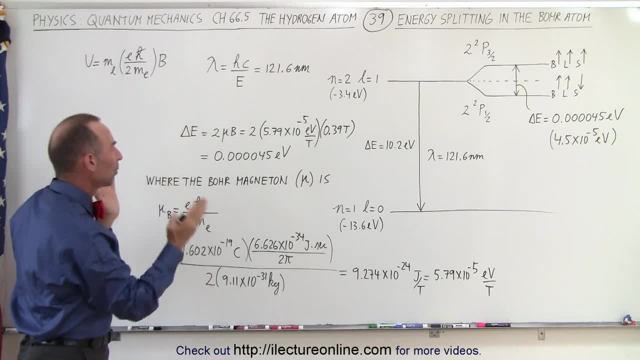 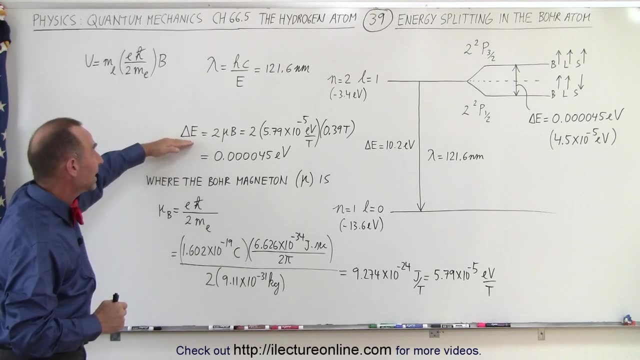 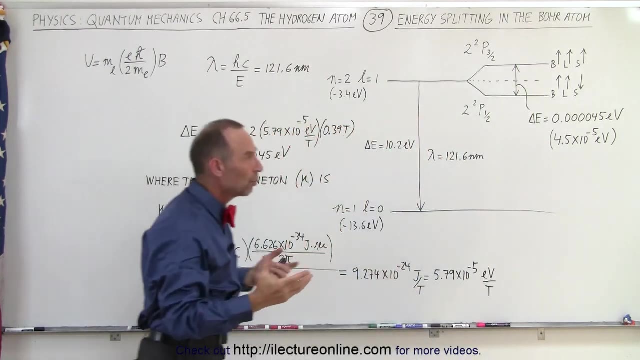 and then this quantity here, which then is what we call the interaction between the spin and that magnetic field, which then produces the change of the energy. Of course, since we have an increase the energy in one direction and a decrease in the energy in another direction, we multiply it times two to get the full value. 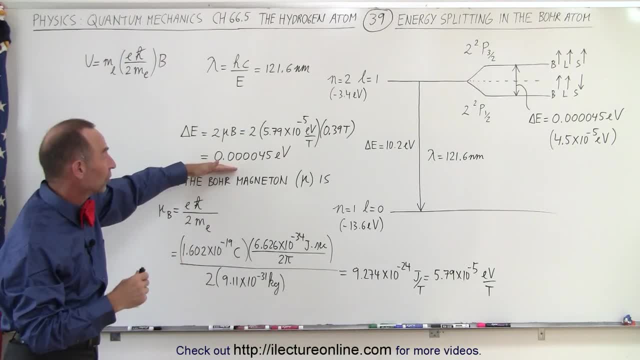 When we multiply these numbers together. this is where the point zero, zero, zero, zero, four, five- did I say enough? zeros? Point zero, zero, zero, zero, four five electron volts, or four point five times ten to the minus five volts. So the Bohr magneton can be calculated as: 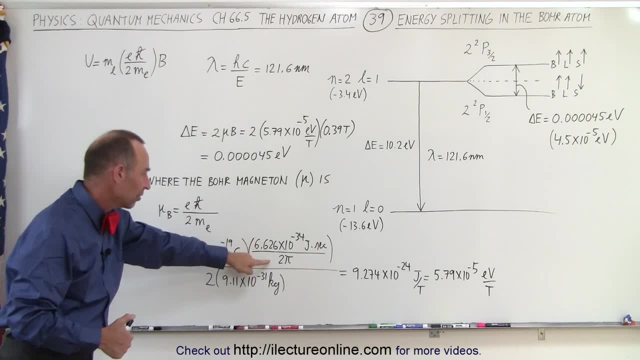 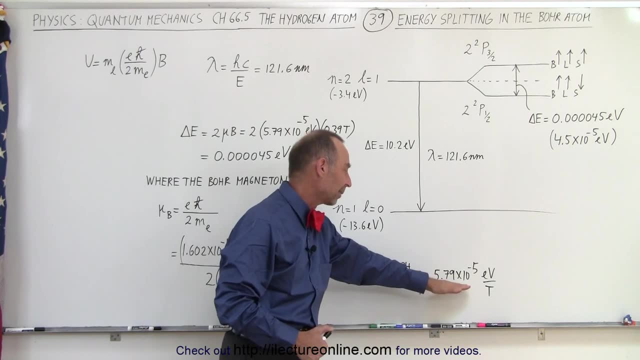 follows the electric charge, Planck's constant, divided by 2, pi divided by 2 and divided by the mass of the electron, which then gives you a value of five point seven, nine times ten to the minus five electron volts per tesla. Notice, that's about the mass of the electron. 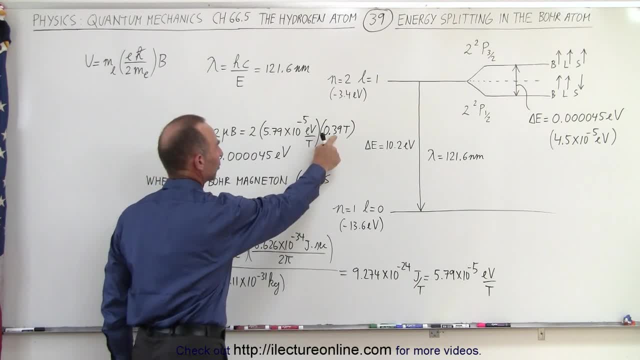 Notice. that's about the mass of the electron, which then gives you a value of 5.79 times the same value, because when we multiply two times point three, nine, we almost get one, and so you can see that when you multiply all that together, you get the value of the difference.